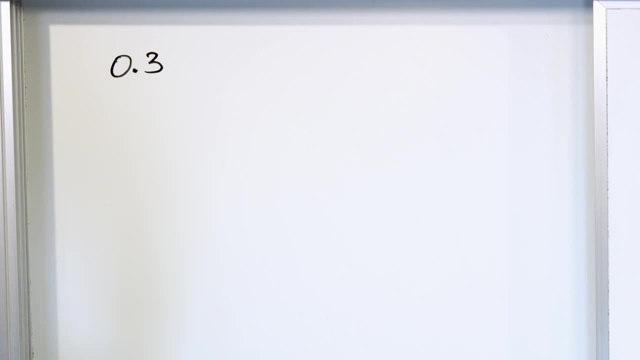 0.3, and I want to convert it to a fraction. a fraction in simplest form or in lowest term. So what does this mean? by the way, The zero means zero wholes. I don't have any whole pizzas or any whole candy bars. I have some fraction and the 0.3 represents 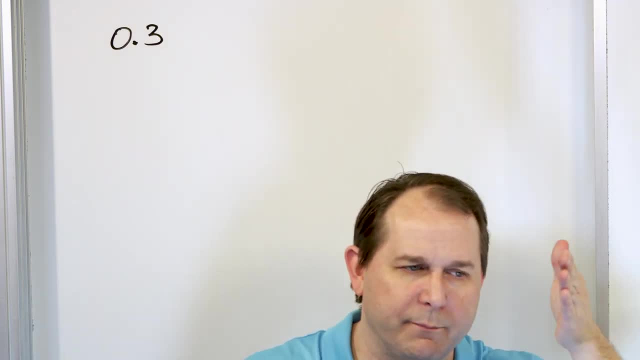 some fractional part, When we get to 0.4, 0.5, 0.6, 0.7, 0.8, 0.9, then we roll over to get one whole candy bar or one whole pizza. So we're really far away from that. We only 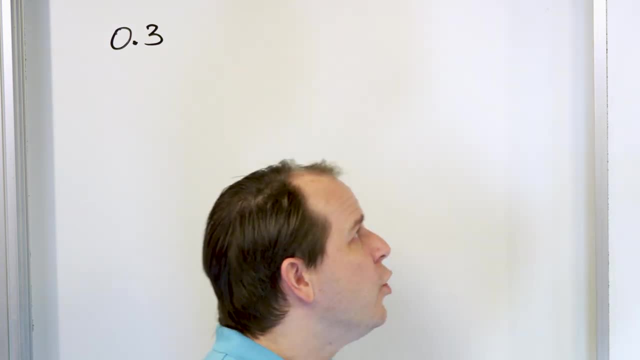 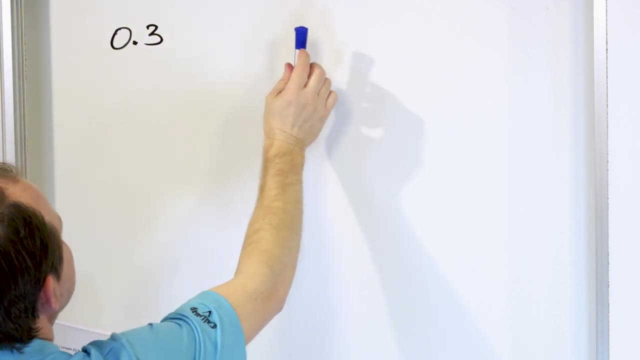 have a small fraction of a pizza right now. What is the fraction? Well, all you have to do is look and say, well, this is in the tenths place because, remember, it goes tenths, hundredths, thousandths, ten thousandths and so on. So to write this as a fraction. 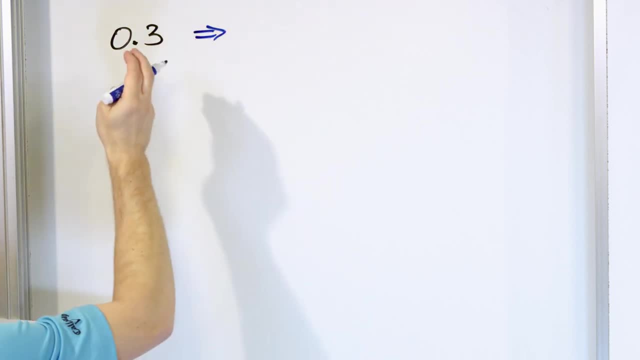 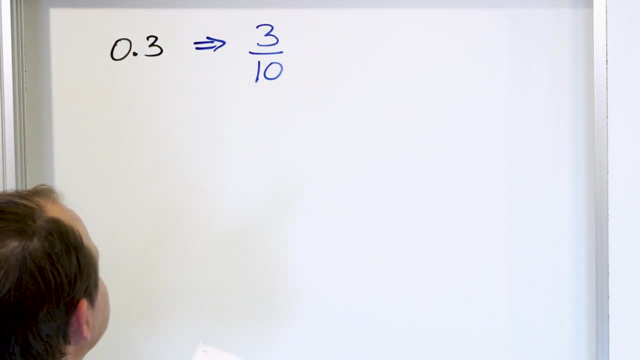 all you have to do is recognize that this is the tenths place. How many of them do we have? I have three of them in the tenths place. It's three tenths. That's actually what this means, And since this fraction is already simplified, I cannot divide top and bottom. 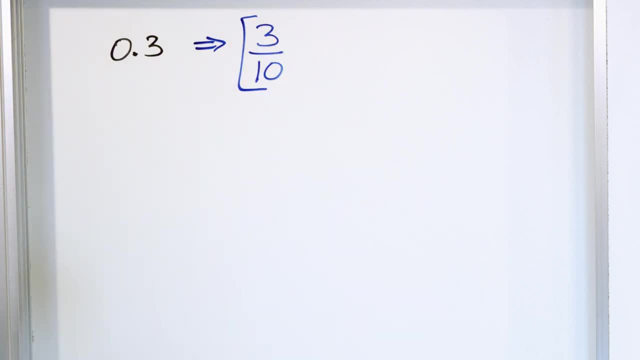 to simplify it further. This is the final answer. So you see, this is a really important example for you to really suck in and internalize it and just think about it. This decimal is telling you everything you need to know about the fractional thing, what it means as a fraction. 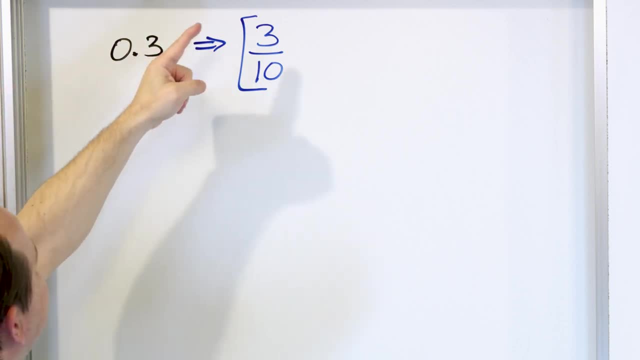 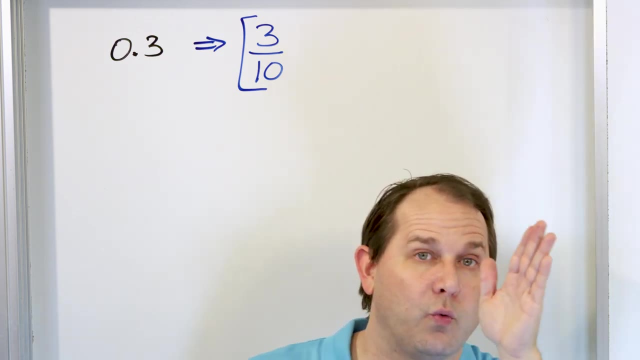 It's in the tenths place. How many do I have Three of them, So it's three tenths. Remember, we can count by tenths. One tenth, then two tenths, then three tenths means I have three little wedges of a pizza E, each shaped to be a size of a tenth. I have three of them, That's. 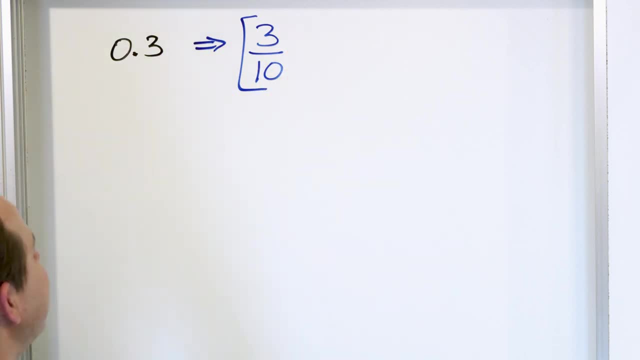 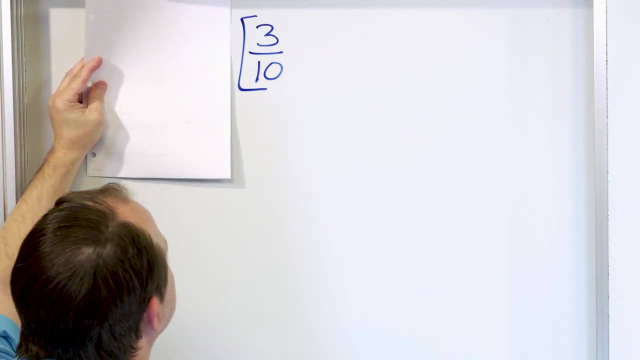 what this actually means. So to write it as a fraction, it's three tenths. If I were to start with this and convert it to a decimal, what would I do, Just from the last lesson, if I said, hey, turn this thing into a decimal. you would say, okay, I'm going to have an invisible decimal. 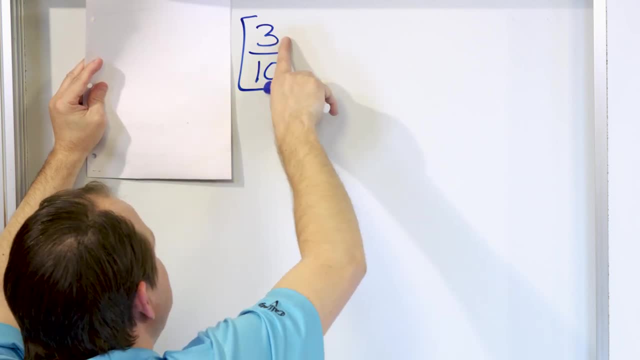 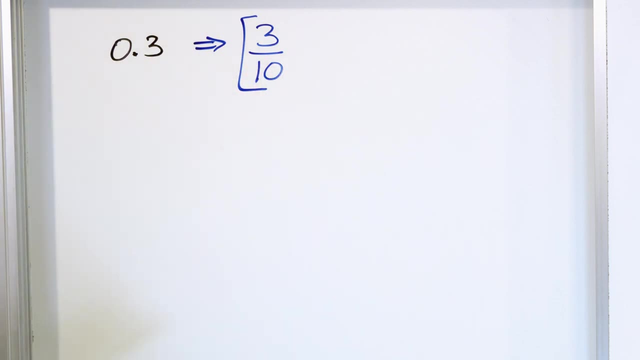 here. I'm dividing by 10, because that's what it is is division. I'm going to move the decimal 0.3. That's exactly it, So you can go either way back and forth and get to the same answers It. 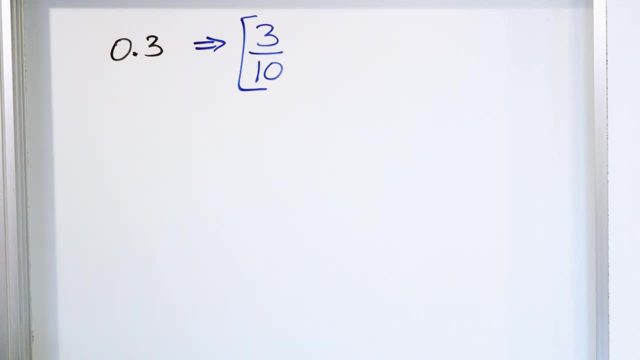 should all work out. If you're doing it all correct, it should all make sense and give you all the correct answers, no matter which way you go. All right, let's take a look at problem number two, if I can ever get there. Problem number two: let's convert the decimal 0.1 into a fraction. 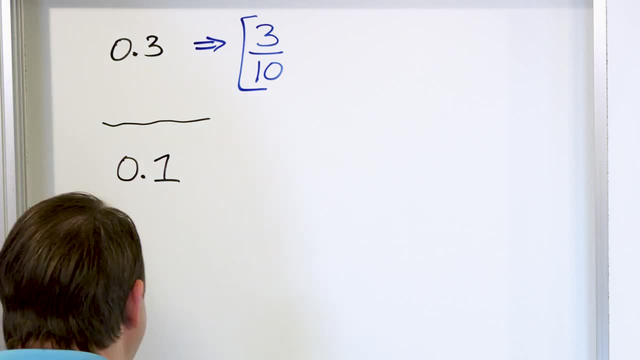 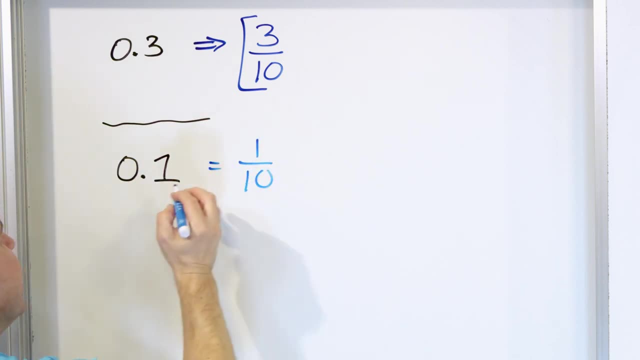 Well, again, this is in the tenths place. So what does it mean to have 0.1?? I have one slice worth a tenth, So I have one tenth. The one goes up here and it's in the tenths place. 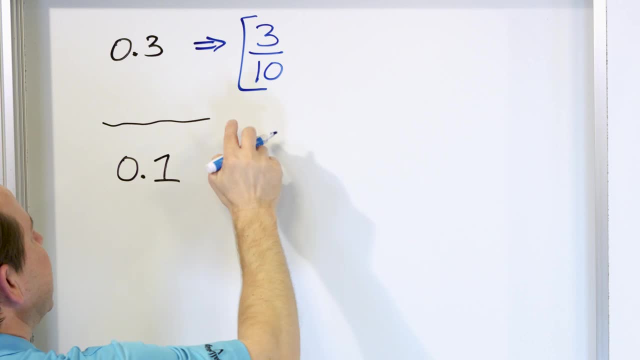 The three goes up there and it's in the tenths place. I cannot simplify this anymore. So the answer is one tenth. Now, if I gave you instead this and said: go backwards, convert this to a decimal, you would divide it. The decimal is here, invisible, and you would move it by dividing by. 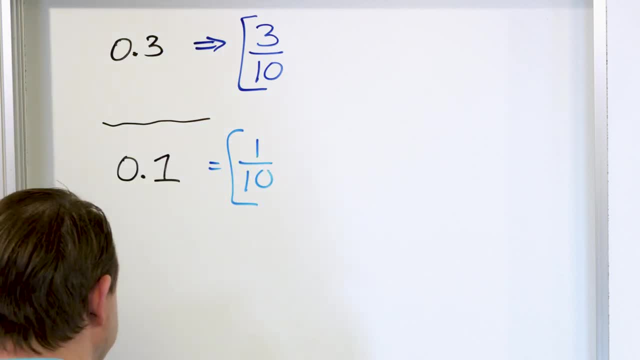 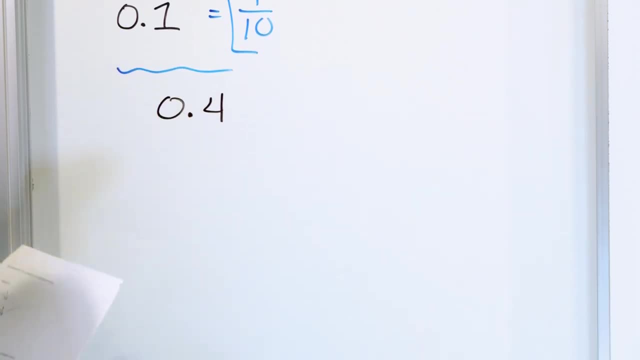 10, 0.1.. That's what we started with, So that's what you have, All right, let's take a look at problem number three: 0.4.. Let's convert that to a fraction, All right. so same story. It's in the tenths place. 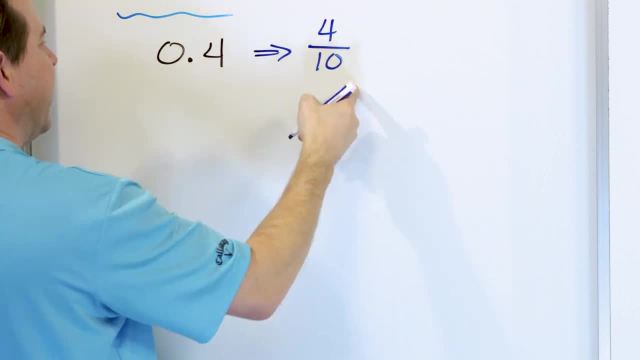 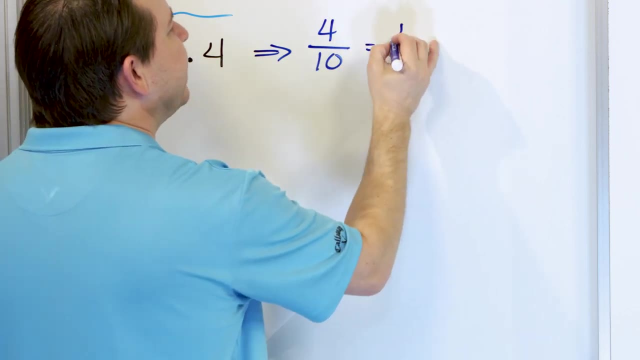 How many do I have Four of them in the tenths place? I have four tenths, Four tenths. That's what that means. But this fraction is not fully simplified. They're both even numbers. I can take the four, I can take the 10, and I can simplify this by dividing by two and dividing by two. 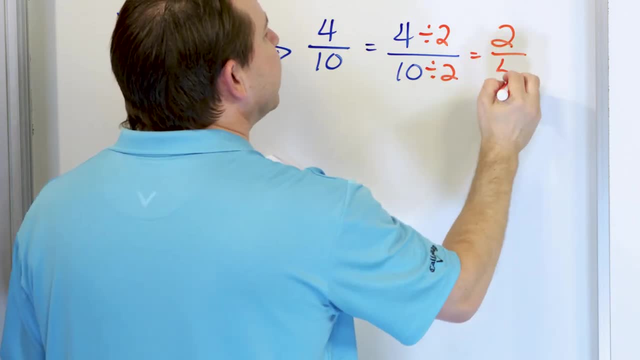 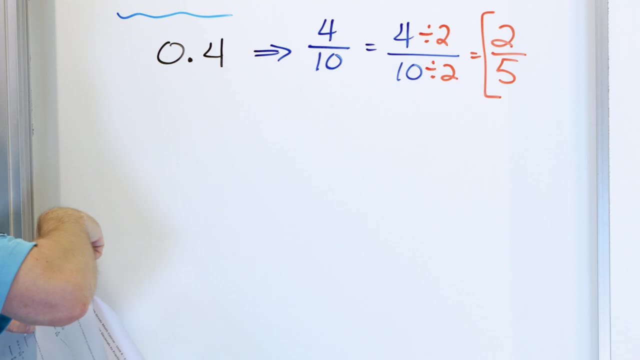 Four divided by two is two. Ten divided by two is five. This fraction is equal to 0.4.. I cannot simplify any further. So this is the simplest fraction, that is, 0.4.. If you go to a calculator and divide two divided by five, this is what you're going to get. If you take four and 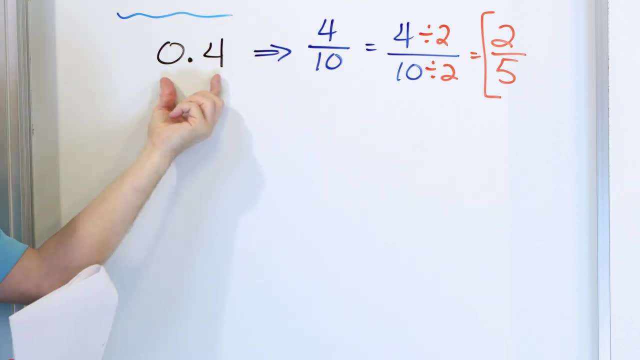 divide it by 10, you're going to get the same thing. This fraction is equal to 0.4.. This fraction is equal to 0.4.. How can that be? It's because these two fractions are the same thing. I've just 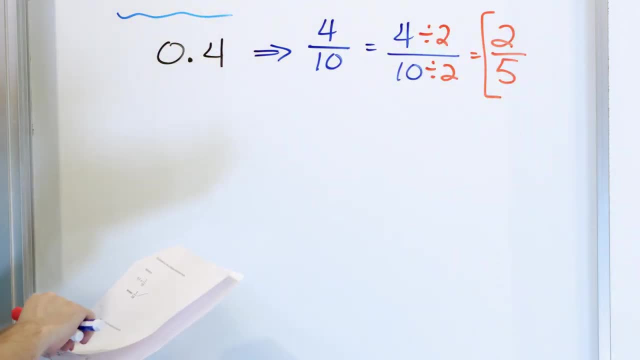 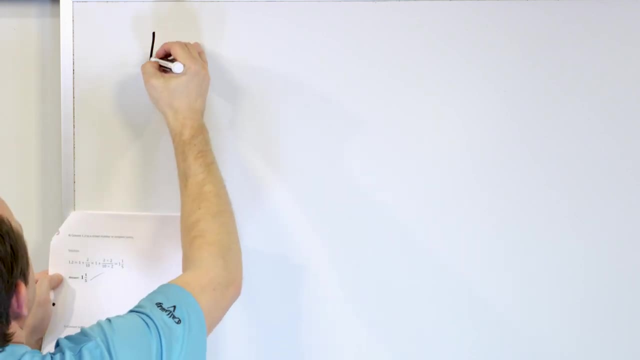 simplified it to something simpler. So when we represent these as a fraction, we always want the simplest form. Let's take a look at the next problem. Let's convert something a little more complicated- 1.2.. Let's turn that into a mixed number 1.2.. What does this mean? It means I have one whole plus. 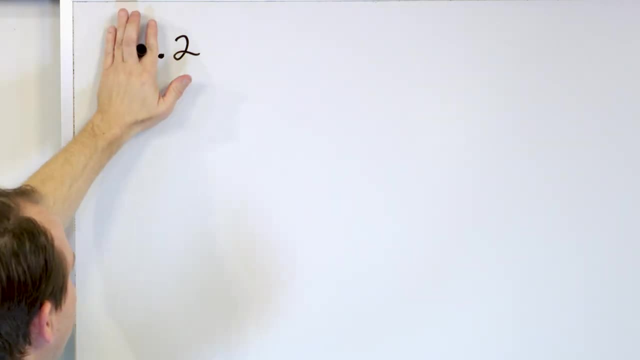 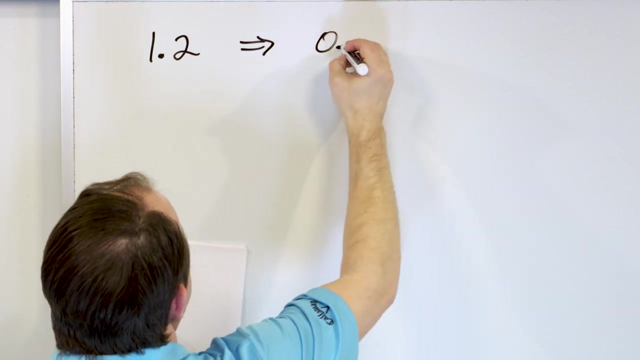 0.2,, which is a fractional part. So let's ignore the whole for now, Only let's look at the 0.2.. The 0.2.. So let's look at this: The 0.2 is what Two tenths right. So this is in the tenths place. 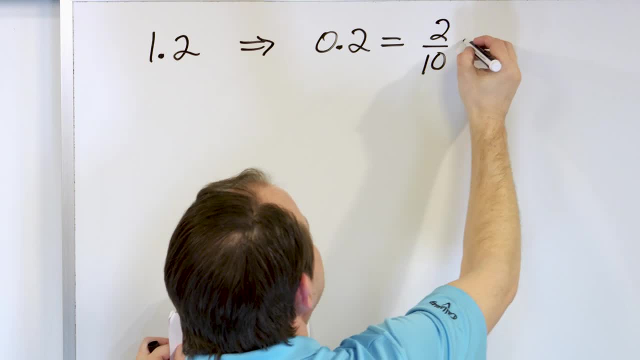 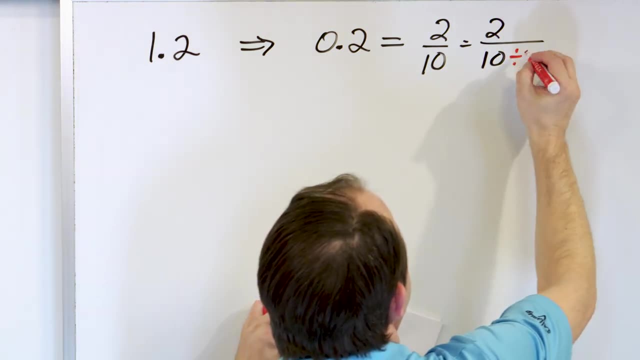 and there's two of them, Two tenths. right Now, can I simplify this any further? Well, 2 on the top, 10 on the bottom. I can divide both top and bottom by 2.. So 2 divided by 2 is 1, and 10 divided by 2 is 5.. So what we? 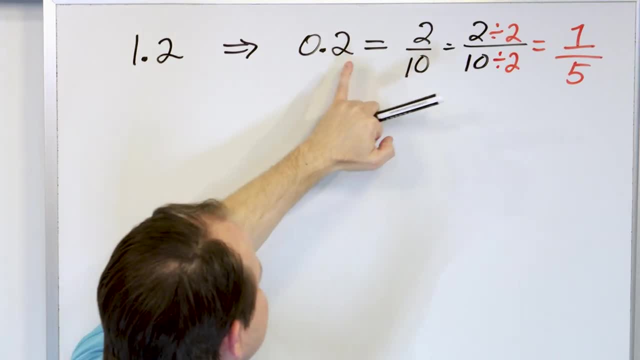 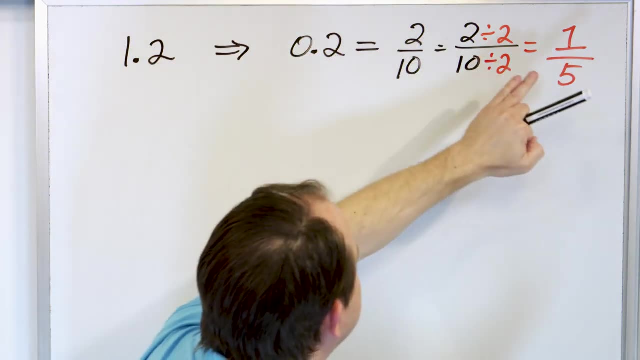 figured out is that the 0.2 part of the problem is equal to the fraction 1- fifth. So that's the fractional part. But the original problem had one whole plus 1 fifth. One whole plus 1 fifth. How do you write that together? 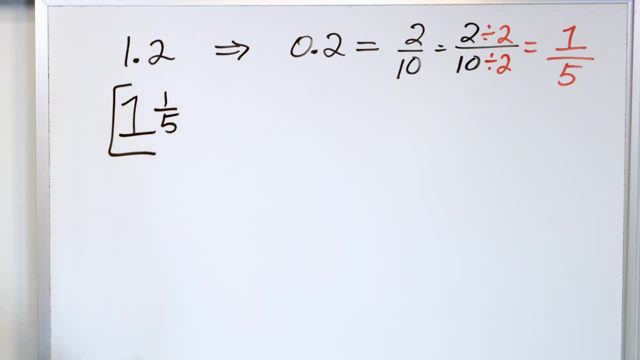 You can write that it's 1 and 1 fifth, So this would be the best way to write it: 1 and 1 fifth. We're converting it into a mixed number. You could write this as an improper fraction if you want. There's. 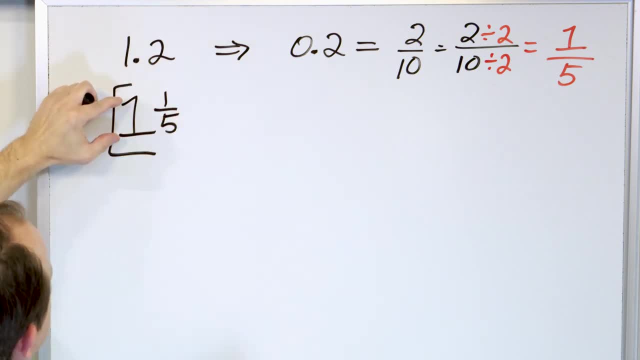 nothing wrong with that, But when you have one whole plus a fractional part, it's very common to write it like this: If you wanted to make it into a improper, you would multiply 1 times 5 is 5, plus 1 is 10.. I'm sorry, 1 plus 5 is 5, plus 1 is not 10.. Plus 1 is 6.. It would be 6 fifths for the. 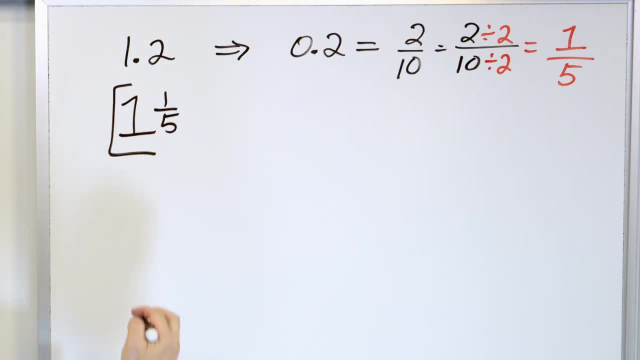 answer there. All right, Halfway done. Let's take a look at 0.002.. That is a decimal. We're going to convert it to a fraction, All right. So what do we do with this? Well, this is the tenths place. This is the 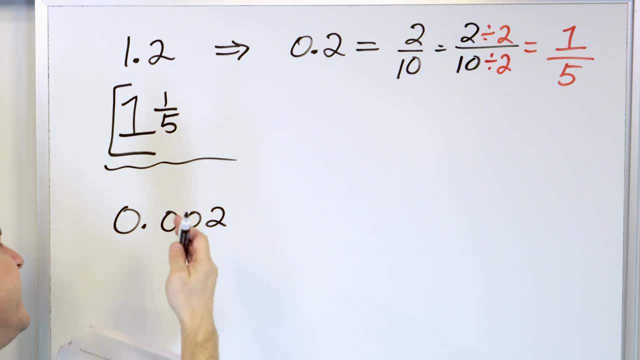 hundredths place. This is the thousandths place. So what is the value of this? I have 2 in the thousandths place. I have two thousandths Right. Not two tenths, because that would be here, Not two hundredths, because that would be here, But two thousandths, which would be 2.. 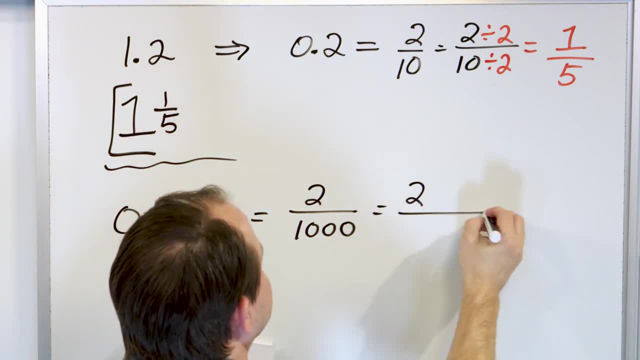 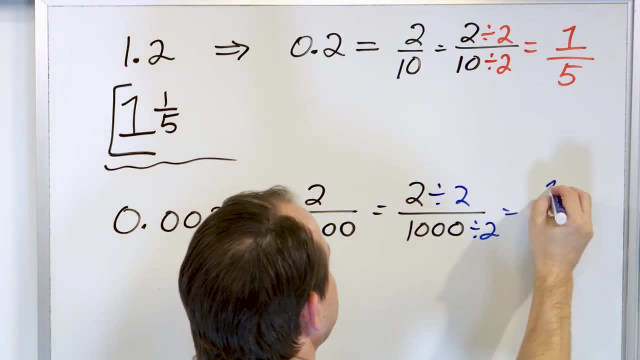 There 2 over 1,000.. How do I simplify this fraction? Well, I can divide top and bottom by 2.. They're both even numbers. 2 divided by 2 is 1.. And what is 1,000 divided by 2? 500.. 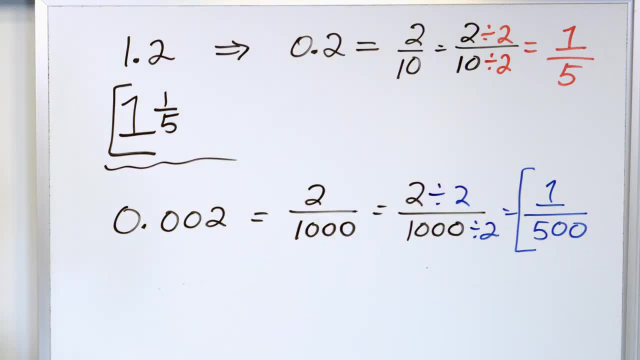 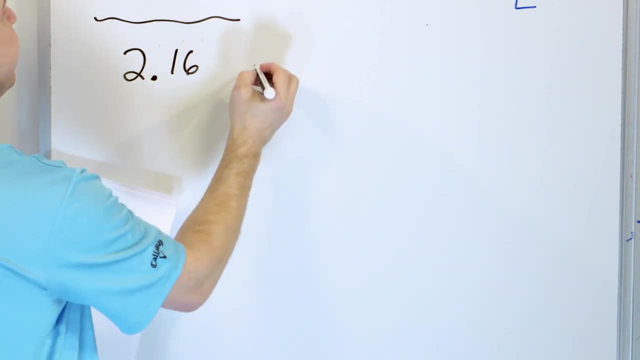 So this is the simplest fraction. that equals 0.002.. 1 over 500.. All right. Next problem: Let's convert the decimal 2.16 into a mixed number. So we're going to ignore the 2.. We're only going to focus on the 0.16.. This is What does this. 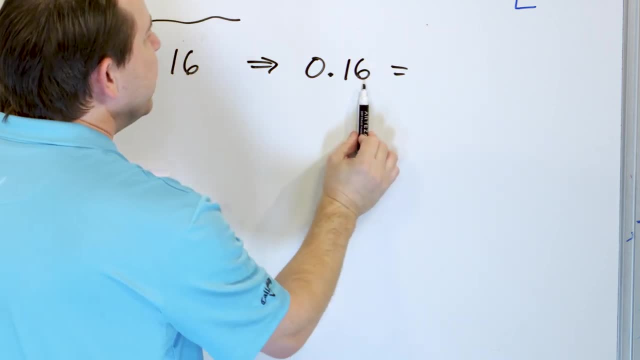 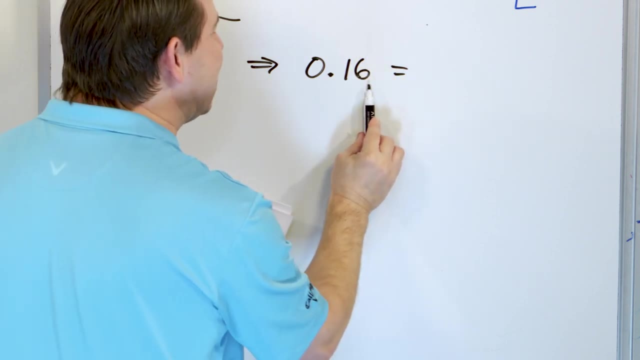 mean This is the tenths place and this is the hundredths place, So I do have 1 in the tenths and 6 in the hundredths, But as a whole together I have 16 in the farthest position over here. 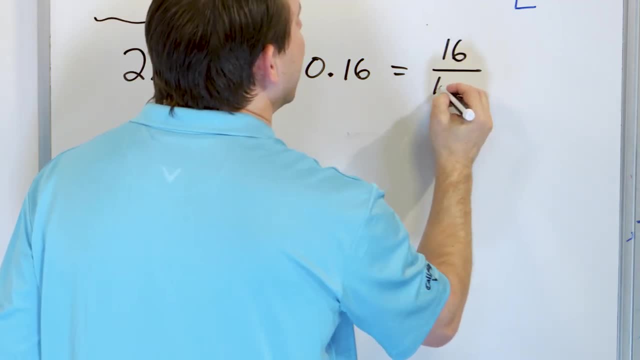 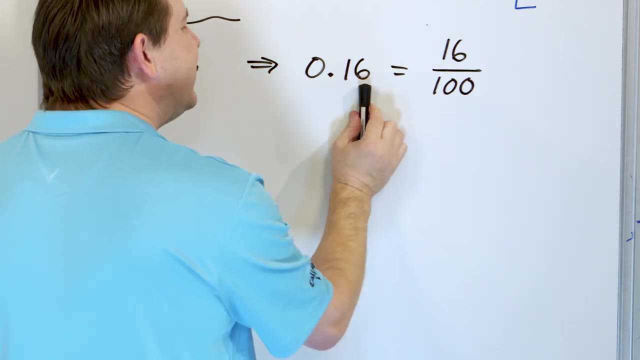 which is the hundredths place, So you write it as 16 hundredths. I want to make sure you understand that, because you do have 1 in the tenths place and you do have 1 in the hundredths place, So I have 6 in the hundredths place, But when you add all those together it's the same as. 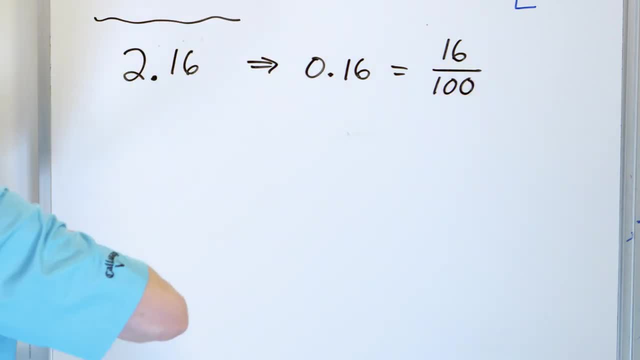 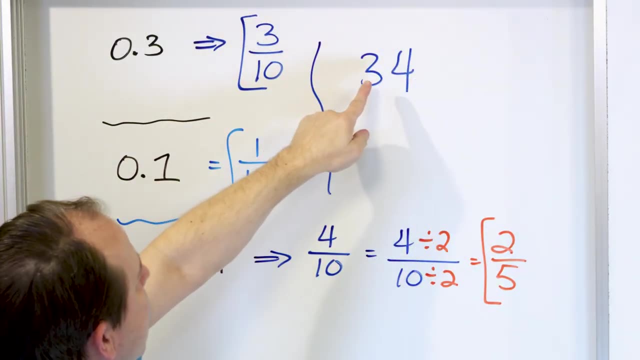 16 in the hundredths place. This is the same thing with regular numbers, by the way. Let's go over here The number 34.. What does this mean? It means I have 3 in the tenths place and I Not the. 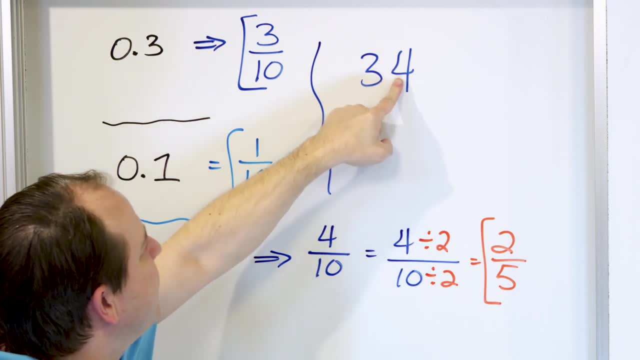 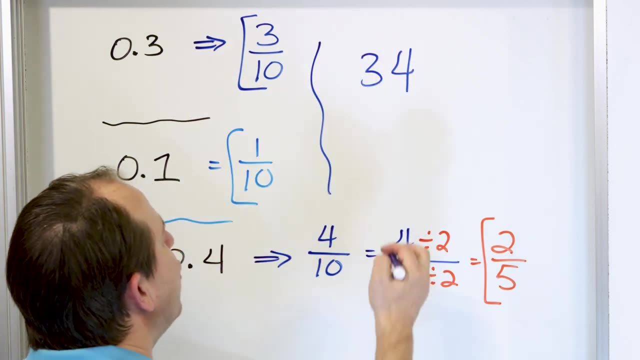 tenths place, The tens place, Three tens And I have 4 in the ones place, But all together we put it together and we say it's 34 ones in the farthest position, 34 ones. What about? 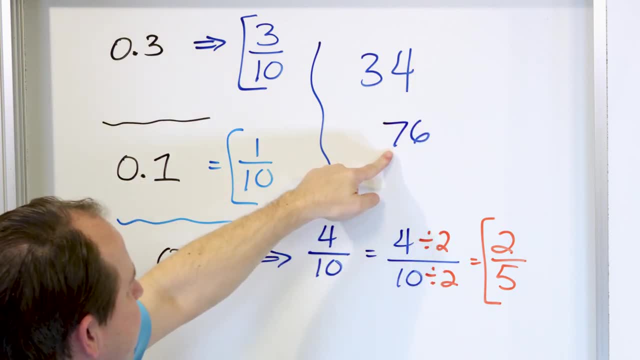 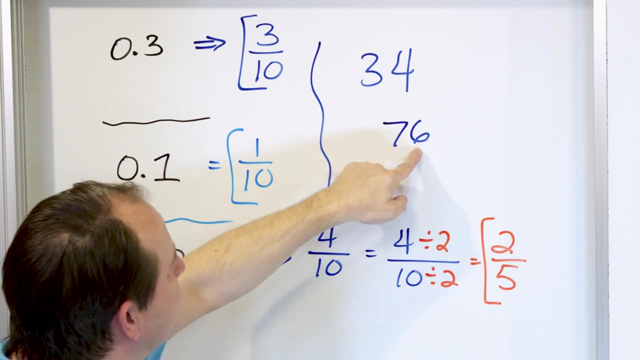 76?? Yes, it's 7 in the tens position for 70.. This is worth 70.. And this is worth 6 in the ones position. So this is worth something in the tens and this is worth something in the ones. But we 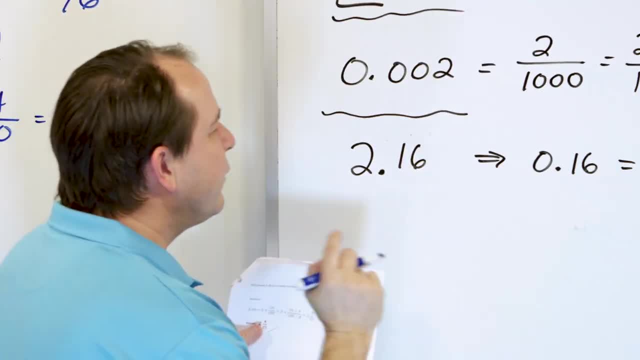 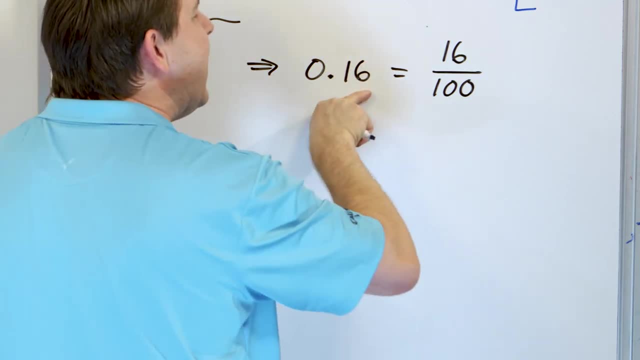 put them together, We say that it's 76 ones, And so here's the same thing. This is 1 in the tenths place, This is 6 in the hundredths place, But all together it's 16 in the farthest position. 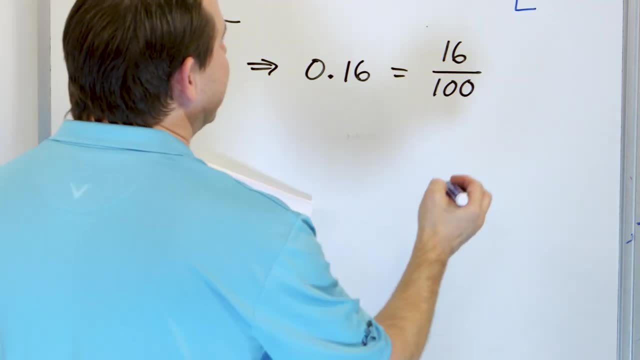 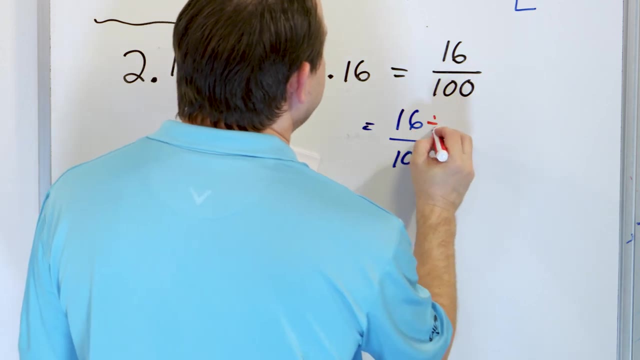 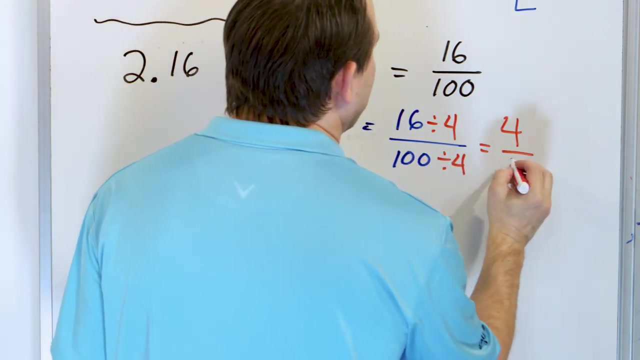 in the hundredths position. So how do I simplify this? 16, one hundredths. What do I do? Well, I know that I can divide the top by 4 and the bottom by 4, because 4 times 4 is 16, so I divide and get a 4.. 100 divided by 4 is 25, and I can't really. 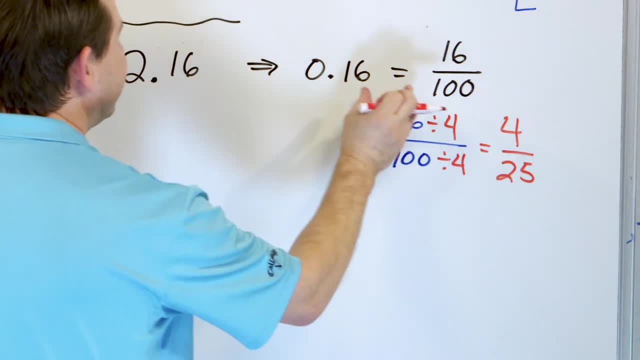 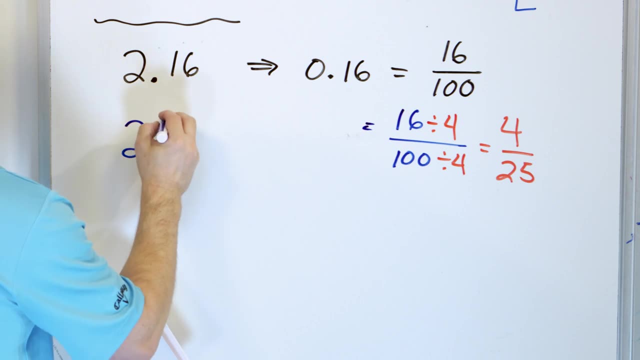 simplify that any further. So I take this fractional representation- That was just talking about the 0.16, and then I attach it to the two holes for 2 and 4- twenty-fifths as a mixed number: 2 and 4- twenty-fifths. If you wanted to do that, you could do that. You could do that, You could. 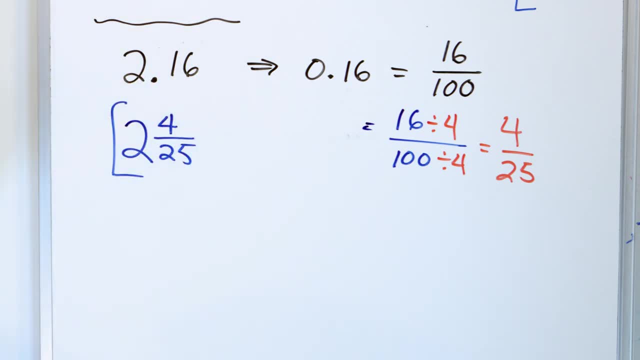 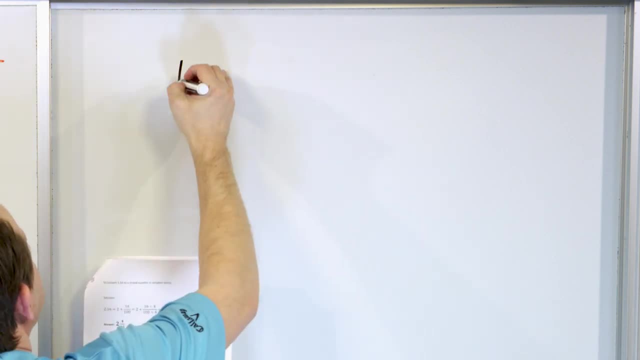 write it as an improper fraction. You could, of course, convert that if you'd like. Alright, we're on the home stretch. Just a few more problems. Let's take a look at the number 1.01, and we're going to convert that into a mixed number. So again, forget about the whole number. 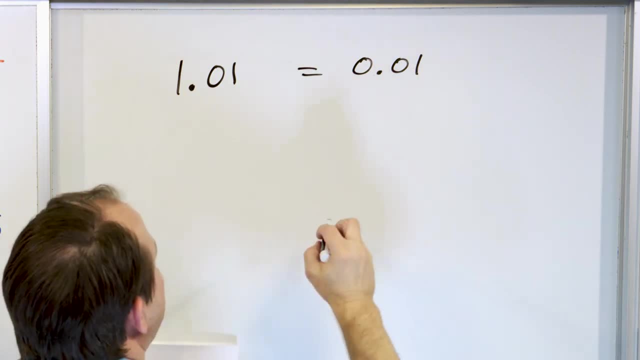 Let's just focus on the 0.01.. So I have nothing in the tenths place, but only 1 in the hundredths place. So I have 1, one hundredth. Alright, that's the fraction. I can't simplify it any more. 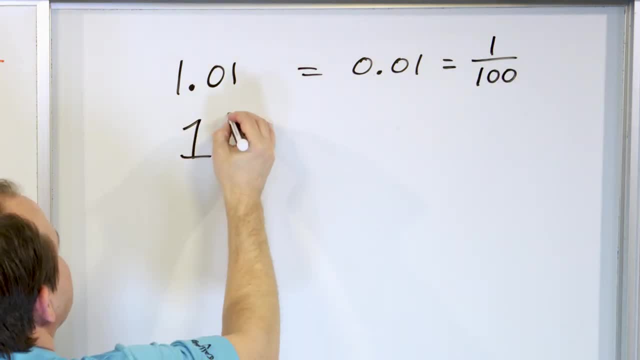 I can't divide top and bottom, so this is it, And I attach it to the 1,. so it's 1 and 1, one hundredth. 1 and 1, one hundredth. That's the final answer. Alright, only three more. Let's take a look at 8.6,. 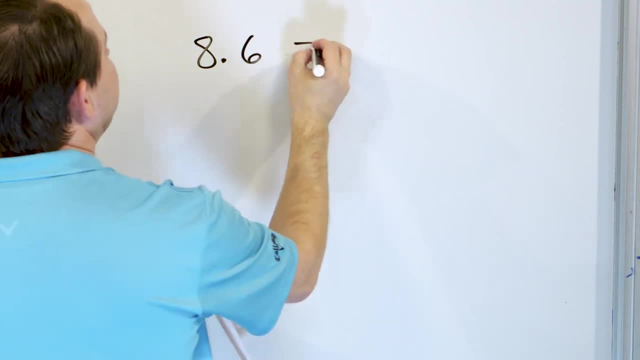 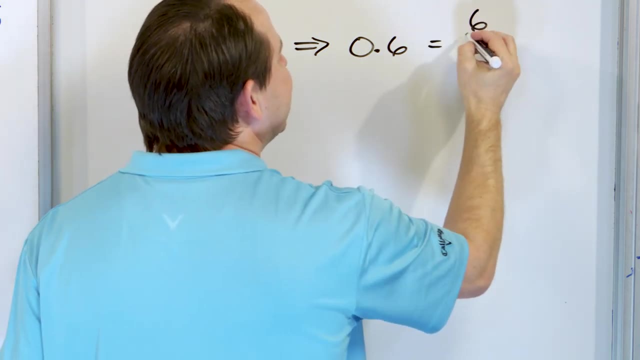 and we're going to convert this into a mixed number. Same thing: we're going to ignore the whole number, We're going to focus only on the 0.6.. And this is in the tenths place. So what does this mean? Six in the tenths place. Now I can simplify this. 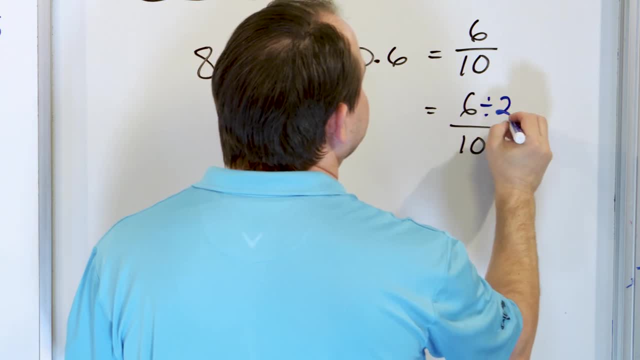 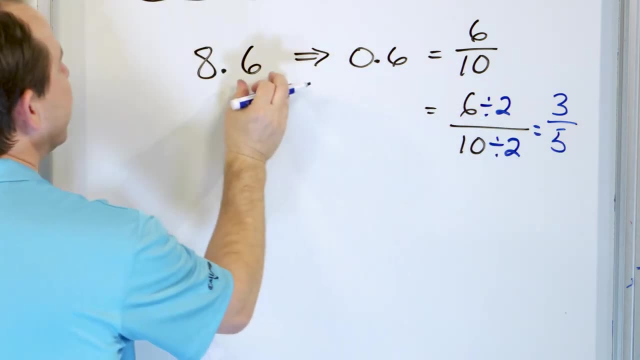 By dividing top and bottom by what? By two? They're both even numbers. And what will I get? Six divided by two is three, and ten divided by two is five. So three-fifths is what the 0.6 means. 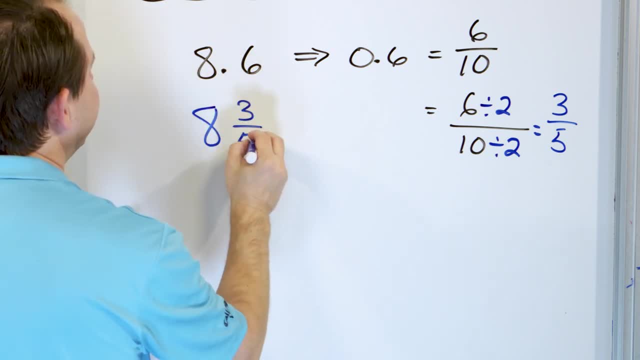 I attach it to the whole of eight, eight and three-fifths. This means eight plus three-fifths, This means one plus one, one hundredth, and so on and so forth. Alright, only two more problems and we're done. Let's take a look at two. 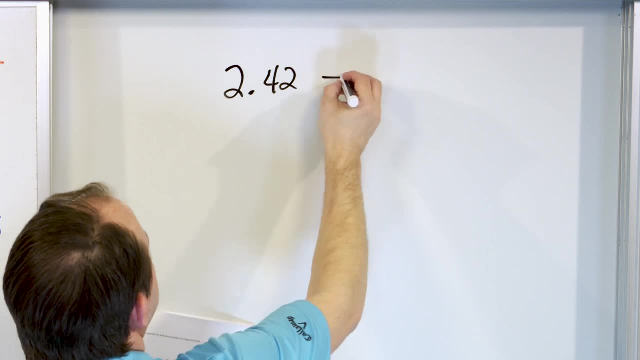 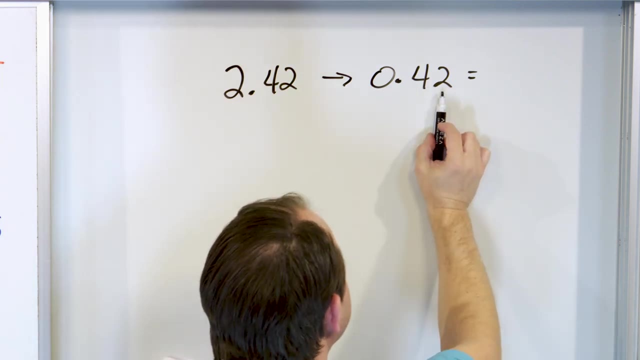 point four. two Convert this to a mixed number. Let's focus on the 0.42.. So, yes, I do have four in the tenths and I have two in the hundredths, But again, taken as a whole, I have forty-two in the farthest position, which is the hundredths place. Forty-two.